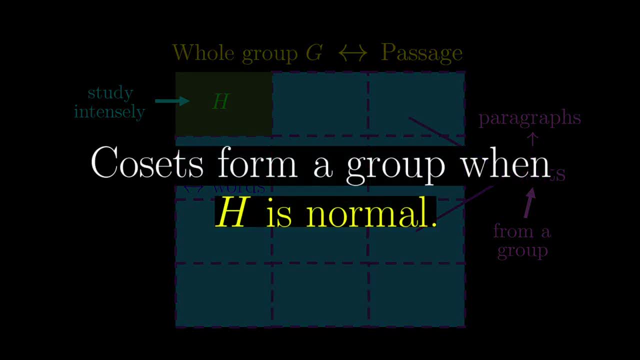 to find out what they are. It turns out that these cosets form a group when H is a normal subgroup, a concept that we have derived together in the last video. For our purposes, these cosets form a group when we can define some consistent operations on the cosets. 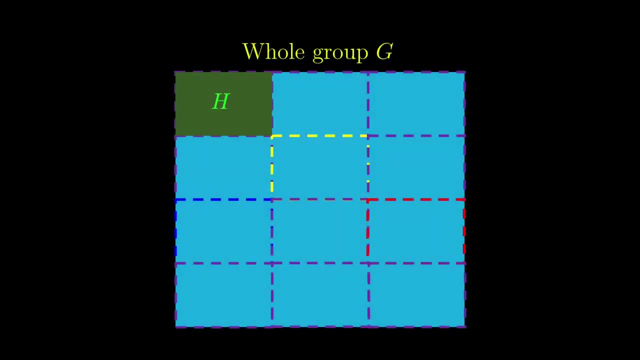 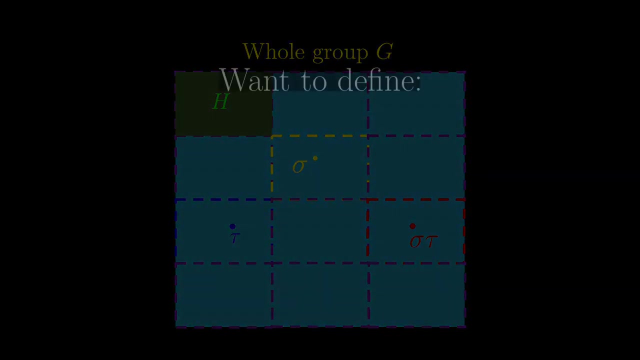 A natural definition of operations on cosets is that if a symmetry sigma is in this yellow coset, another symmetry tau in this blue coset, and the symmetry sigma tau lies in the red coset, then we want to define yellow coset dot blue coset 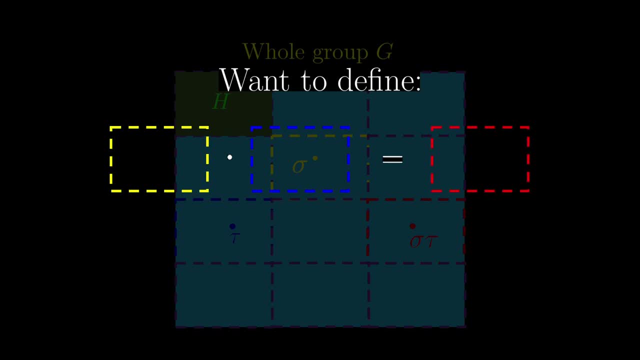 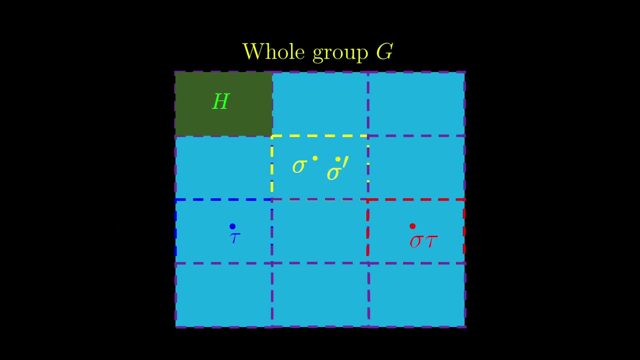 to equal red coset. Again, notice that this is not normal multiplication in the sense that we do not necessarily have blue coset dot yellow coset to be the red coset. In other words, order matters, like normal symmetries. For a general subject, we can use the same formula for the symmetry sigma subgroup H if we pick sigma prime from the same yellow coset, tau prime from the same blue coset 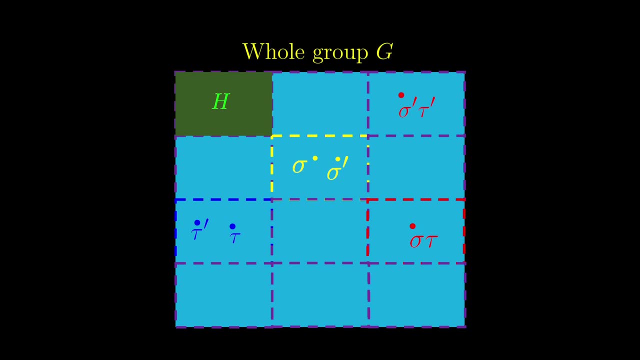 instead, sigma prime tau prime might end up elsewhere. Of course, we want it to lie in the 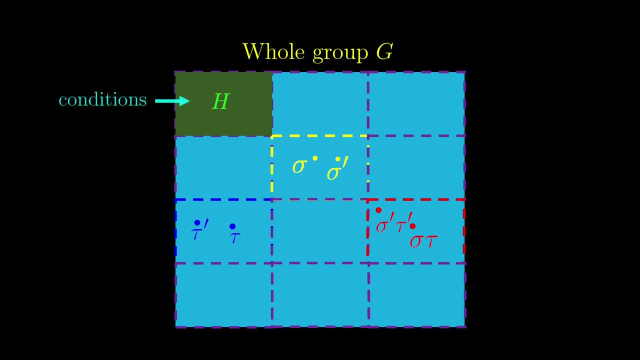 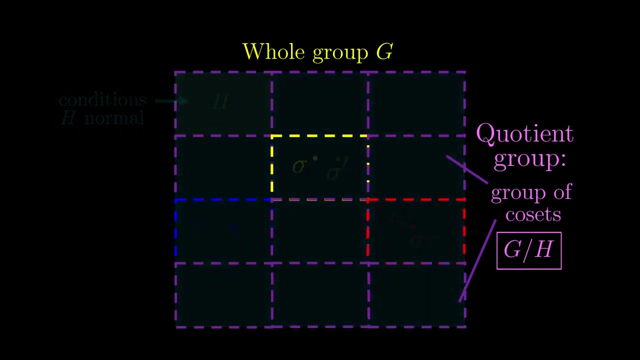 red coset for consistency, so we need to impose some conditions on the subgroup H. These conditions turn out to be that H needs to be normal. The resulting group of cosets is called the quotient group, denoted G forward slash H, and read as G mod H. This is a more abstract concept 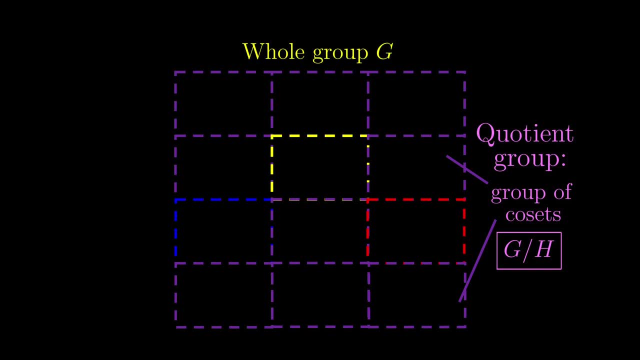 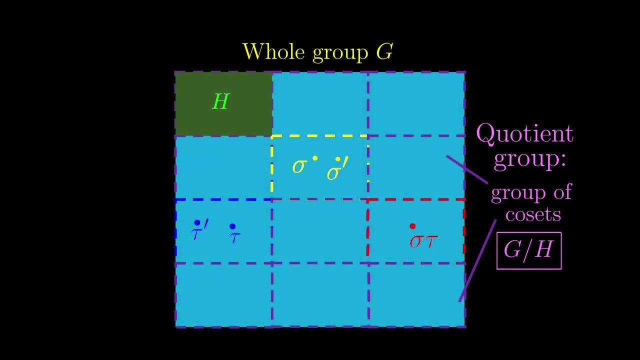 because it is not a group of symmetries anymore, it is a group of sets, which themselves contain a lot of symmetries. But wouldn't it be nice if we can still kind of treat these sets like symmetries? This yellow coset acts very much like sigma itself in terms of operations, and the blue coset acts very much like tau itself in terms of the quotient group. So maybe we can just call this yellow coset sigma, and this blue coset tau. Actually, mathematicians do that, just that we stick an H at the end to remind ourselves that this is not just a symmetry, 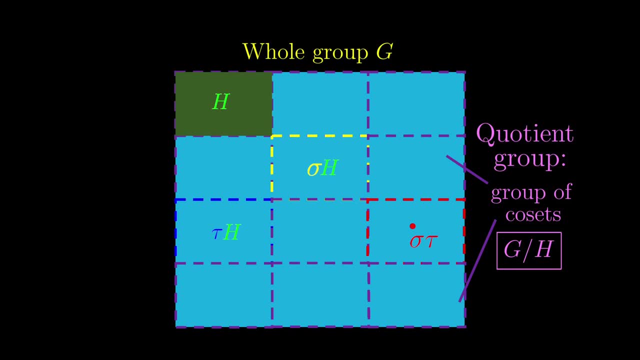 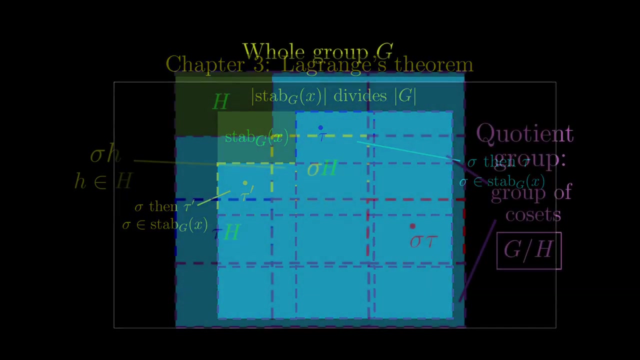 but a coset. This notation actually comes from our definition of a coset, for example, this yellow coset is just a collection of symmetries of the form sigma H, where little h is in the subgroup H. This definition was introduced in the context of stabilisers in chapter 3 of this video series. But there is something special for quotient groups. 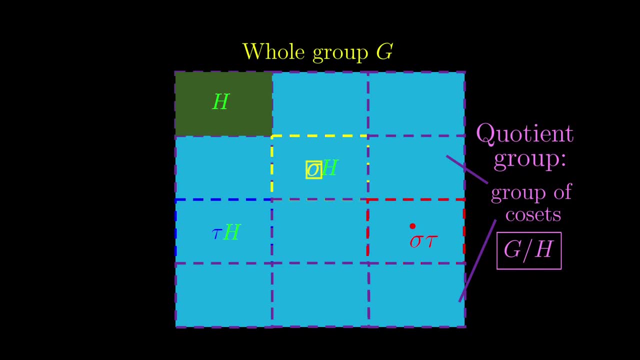 You can choose anything inside the yellow coset in place of sigma, and it does not affect the operations of the cosets within the quotient group. Same for tau. 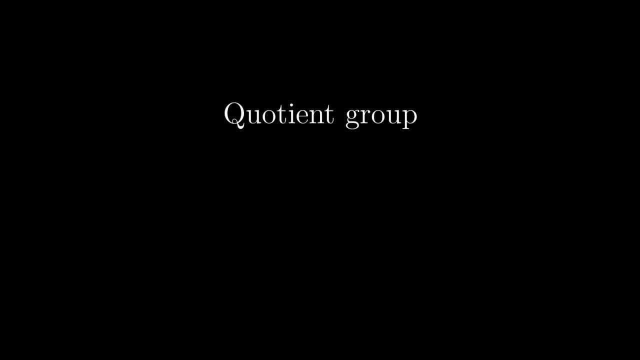 The quotient group is the most popular name for this concept. However, there is another name called the factor group. However, I myself like to think of it as a group of remainders. 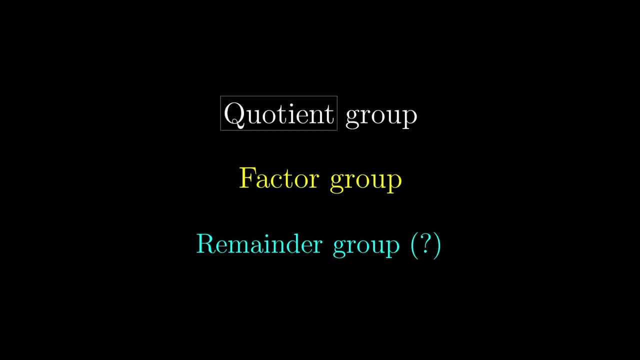 You probably just need to learn one name and be stuck with it, but knowing why there are different names helps you build better intuitions on what a quotient group really is. 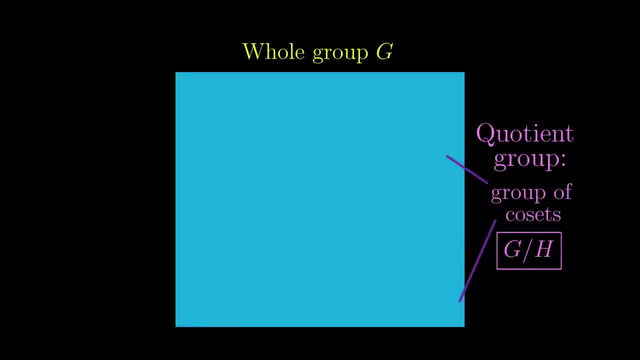 It is not very difficult to make sense of why quotient groups are named this way. We basically divide the group into a collection of cosets, so the act of division is definitely related to quotients here. A more direct way to see this is by Lagrange's theorem. Here, the number 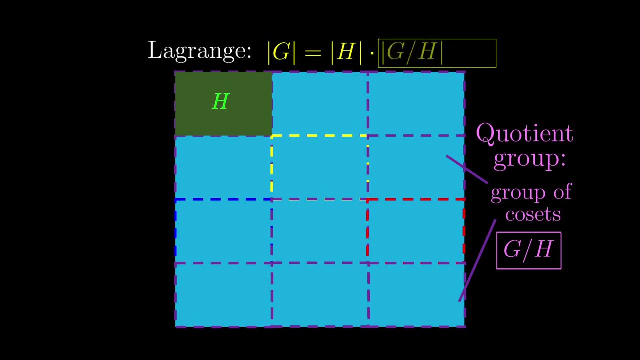 of cosets is just the size of this quotient group by definition. By simple rearrangement, we can see that the size of the quotient group is really the quotient when the size of the whole group G is divided by the size of the subgroup H. Another perspective starts off with this yellow coset containing the symmetry sigma. As said before, the coset contains all elements of the form sigma H, where H is in the subgroup capital H. Here, sigma looks like a factor, 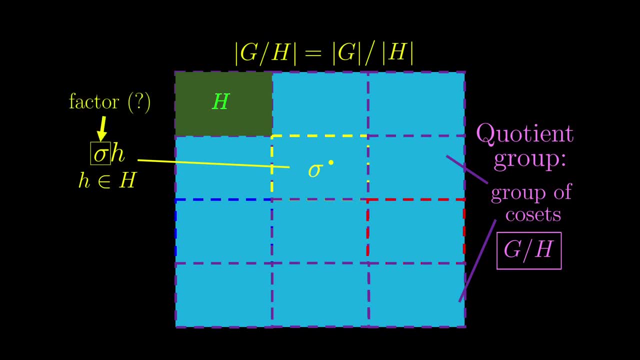 because the notation here looks like normal multiplication, so the set of cosets can be seen as just a group of these factors. What about thinking of this as a remainder group? This 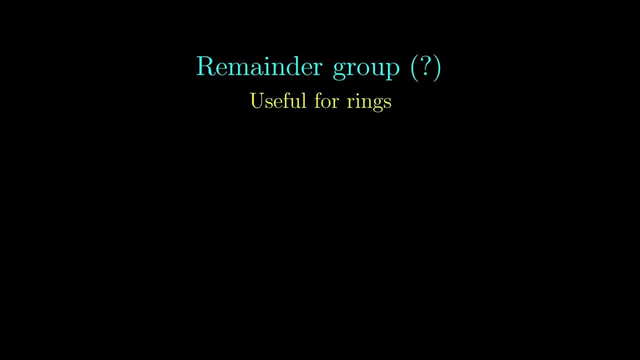 intuition is particularly useful when we are dealing with rings, a specific type of groups. The rings we consider will only be the set of integers z, and the set of real numbers, r, as they can be visualised as symmetries. More specifically, each integer or real number can be thought of as translational symmetries of the number line. For example, the integer negative 2 can be thought of as the translational symmetry to the left by 2 units, and the real number pi can be thought of as the translational symmetry to the right by pi units. 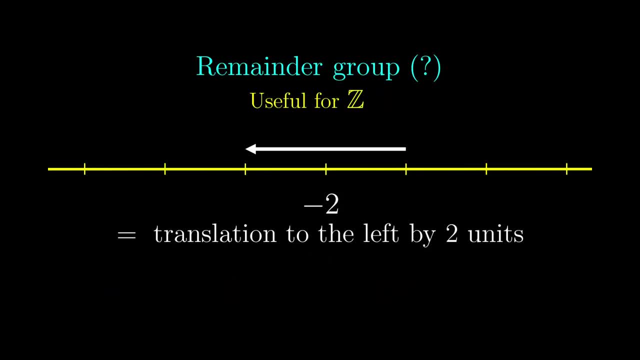 We will focus only on integers, where we can talk about remainders. 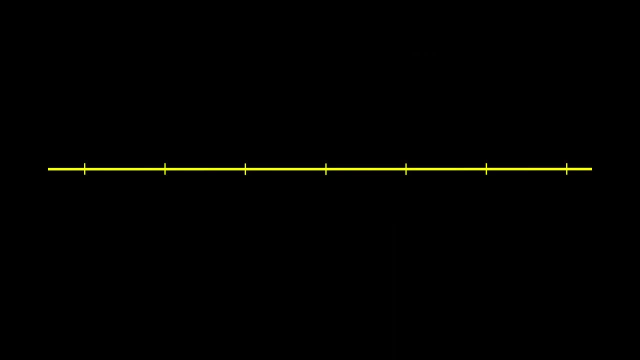 The notations for group operations for this group are a bit tricky. In the previous chapter, we say that if there is a symmetry corresponding to G then H, where G and H are both symmetries, we will call the symmetry HG, simply concatenating the symmetries. However, if we are considering the set of integers as translational symmetries, simply concatenating does not make sense. For example, if we do negative 3, then 2, then simply concatenating the symmetries looks like we get the result to be negative 6. This is obviously not true. Translating to the left by 3 units, then translating to the right by 2 units is equal to a translation to the left by 1 unit, i.e. negative 1, not negative. An obvious patch to this notation would be to attach an addition sign between the two symmetries, and this will then make sense in our example. But this is the only time we don't simply concatenate 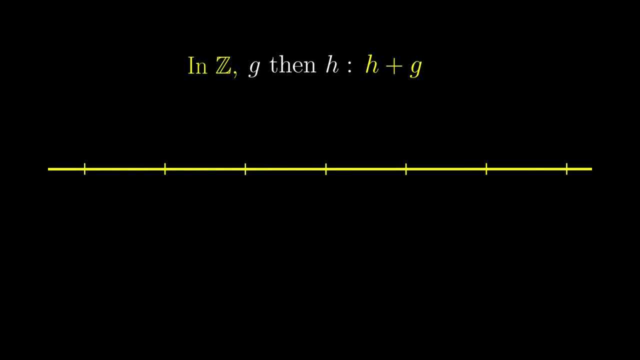 symmetries. Another notation that we need to talk about is undoing symmetries. 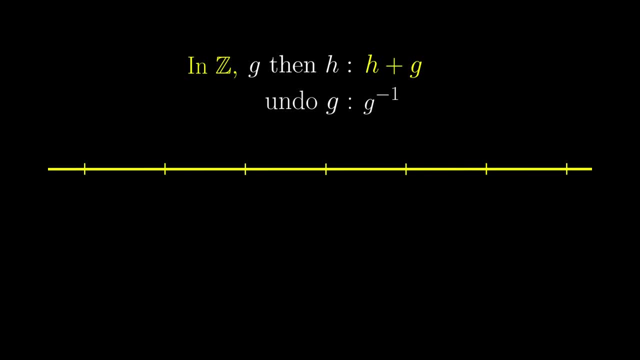 We denote this by G to the power negative 1. Again, if we apply this to this situation, we get some nonsense like 2 to the power negative 1, which isn't even an integer. 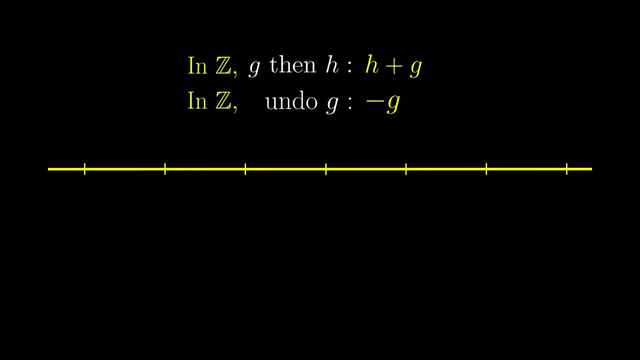 The patch here would be to just stick the negative sign in front of G. 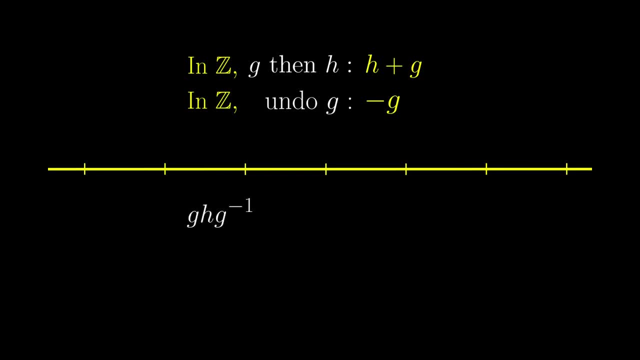 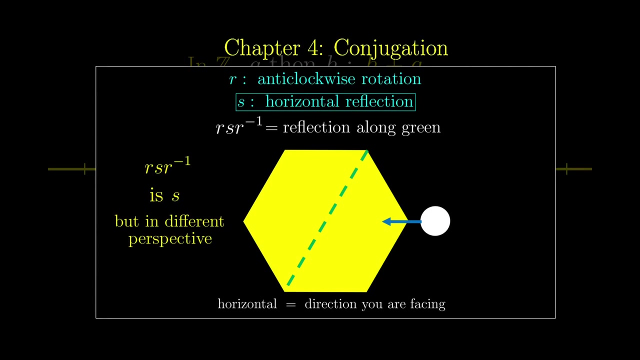 So if we consider the conjugation of H by G, it should change to G plus H, plus negative G, because instead of concatenation, we add plus sign between these symmetries, and the inverse symbol is replaced by the migration. Speaker, even if we want to measure musicians and musicians who dobrze inteligente could work brilliantly with a organizational rule, we just stop at the proper and minus sign. By our usual arithmetic, we have this to be simply h itself. You can also see this more intuitively by our conjugation intuition introduced in chapter 4 of the video series. 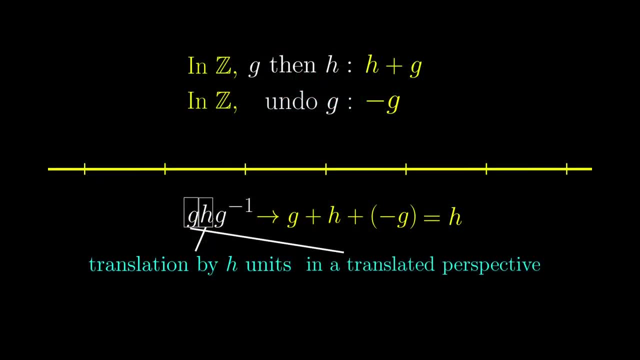 Conjugation means the symmetry h, viewed in the perspective stated by the symmetry g. In whatever translated perspective, it is going to be the same translation by h units anyway. All this is to say, conjugating h by anything is still h itself. A natural consequence of this is that for any subgroup h, conjugating by any symmetry g would be equal to the subgroup h itself, which means that all subgroups of z are normal. For z, it is similar to z beline for anything that does not contain the symmetry g. Eating 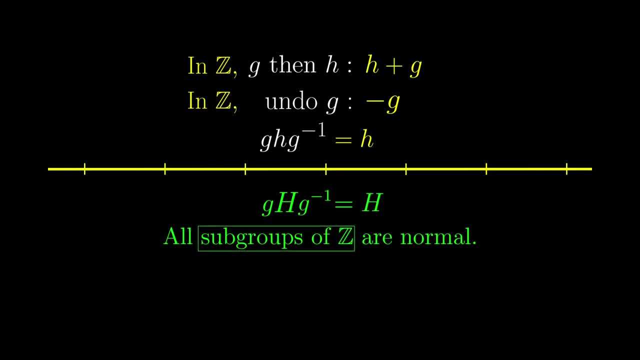 z, we can actually write down the form of the subgroups. We usually denote these subgroups as nz, which means the set of all multiples of n. Since nz is a subgroup of z, it is also normal, which means we can consider the quotient group z mod nz. 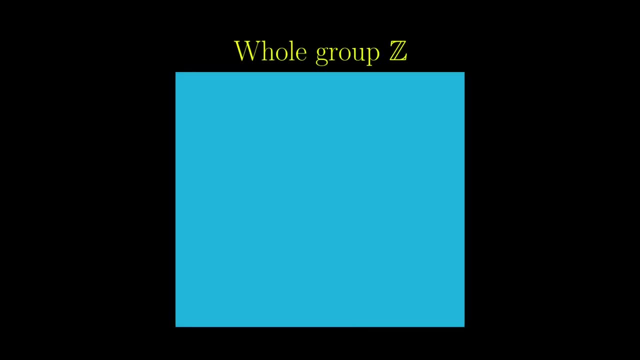 Consider this diagrammatic representation of z. Let's consider a subgroup of z, which is 12z. We just pick n in the previous discussion to be 12. Now 1 is outside this subgroup because it is not a multiple of 12, so this is why we can then construct a coset with 1 in it. We call this coset 1 plus 12z, because one of the elements is 1, and the subgroup in consideration is 12z. And again, instead of simply concatenating the symmetry with the set of n, we just pick n in the previous discussion to be 12. Now, since we have 1 and the subgroup 12z, we add an addition sign here to avoid confusion. Similarly, 2 is not included in 12z or 1 plus 12z, so we can then form another coset, which is similarly named as 2 plus 12z. 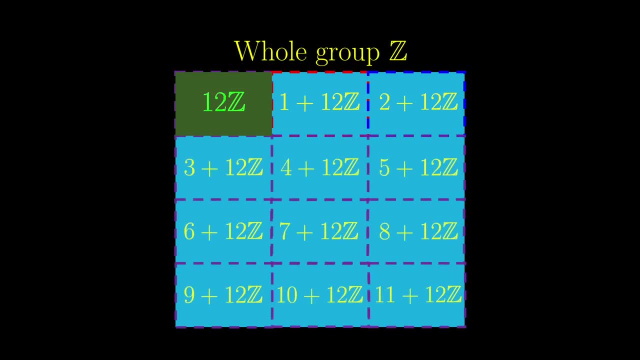 Very similarly, we can construct all the other cosets of 12z, and we can cover the whole set of integers. 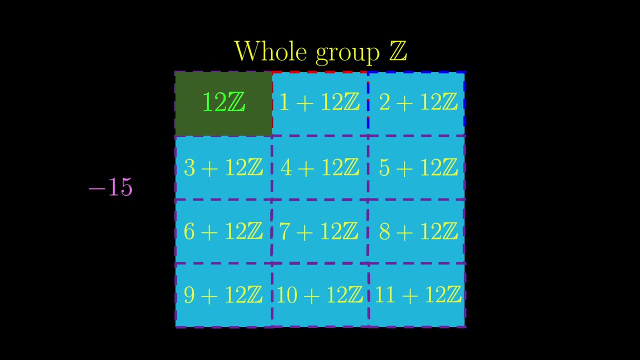 For example, we want to work out where negative 15 lie. Since it is equal to 9 plus negative 24, and negative 24 is a multiple of 12, it must be in this coset, 9 plus 12z. In fact, this 9 here is just the remainder, when negative 15 is divided by 12. So this z mod 12z can really be viewed as just a group of remainders. The next two are equal to 9 plus 12z, and negative 24 is just a group of remainders, 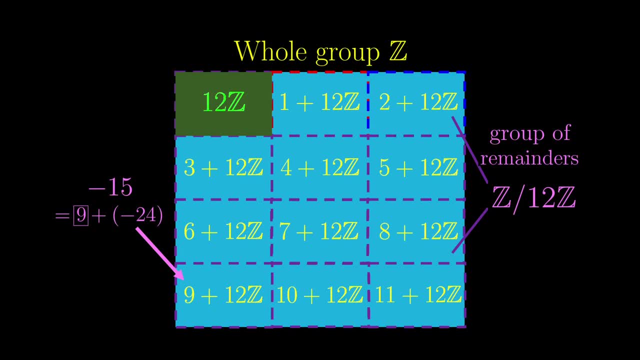 when divided by 12. As a side note, this is one of the formal definitions of operations in modular arithmetic, at least for addition. 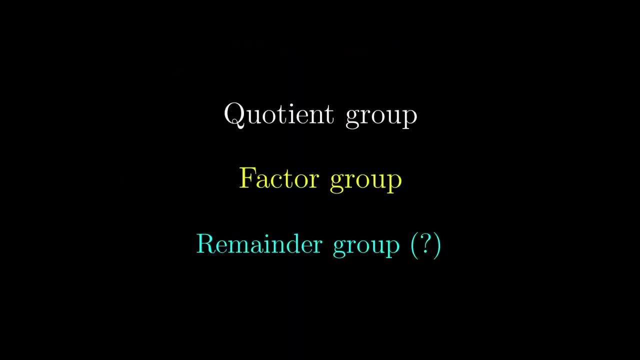 So now you have seen how the quotient group can be thought of in different ways, which hopefully builds up better intuition for this crucial concept. The next video will be about 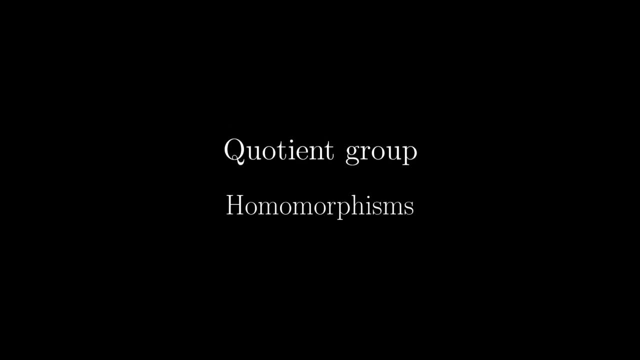 group homomorphisms, which gives paramount importance to quotient groups. If you think that this was helpful, don't forget to like and subscribe! If you liked this video, please 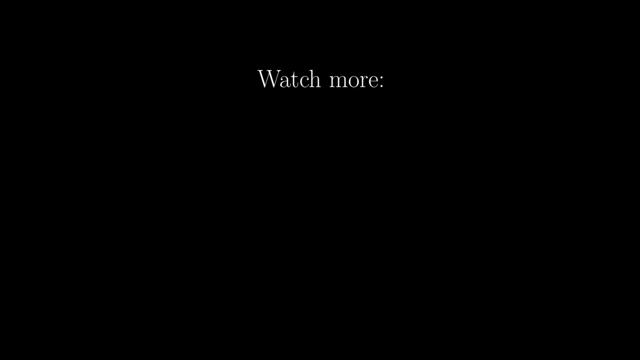 If you think this video series is useful, give it a thumbs up and share it. Don't forget to subscribe with notifications on to stay tuned to this video series. See you next time!